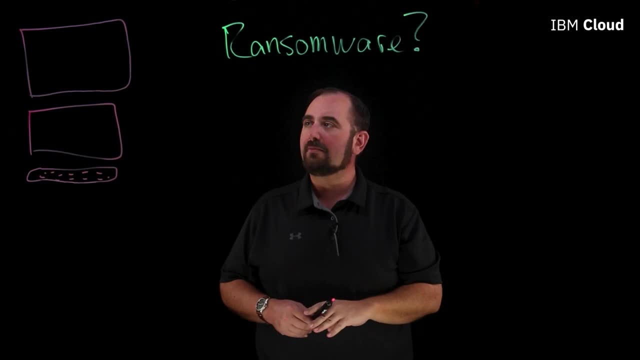 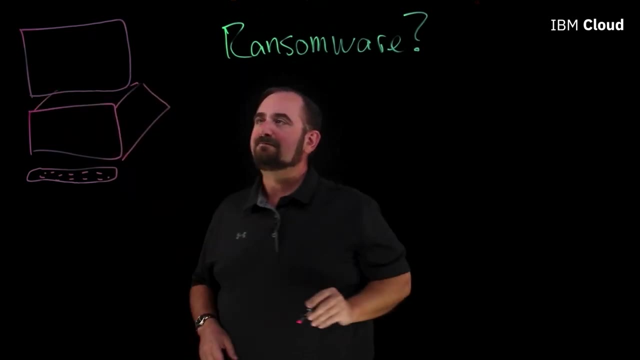 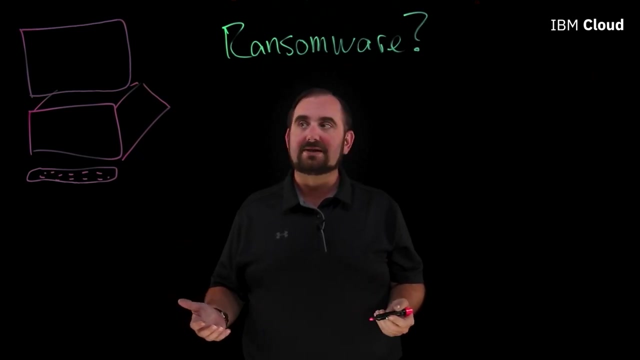 We've got our keys on the keyboard And our computers humming along right, We're doing our computer things, doing everything that we need to, And in the operating system there are always going to be security vulnerabilities of various kinds. It's just inherent to computing. We are never going to find every bug. The best we can do is, as we find bugs, we fix them. But these security vulnerabilities can be exploited, right. 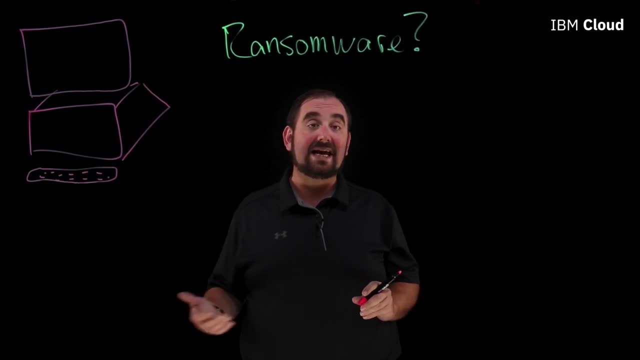 There are large groups of malicious actors out there that are constantly scanning, looking at code, looking for these vulnerabilities, looking for the ability to access systems. So when one of these vulnerabilities is discovered, what a malicious actor will do is they'll figure out. all right. first of all, is this protected against? If it's not protected against, how can I exploit this? How can I use it to make money? Because, at the end of the day, these malicious actors- most of them- aren't doing it for fun. They're doing it to get money. 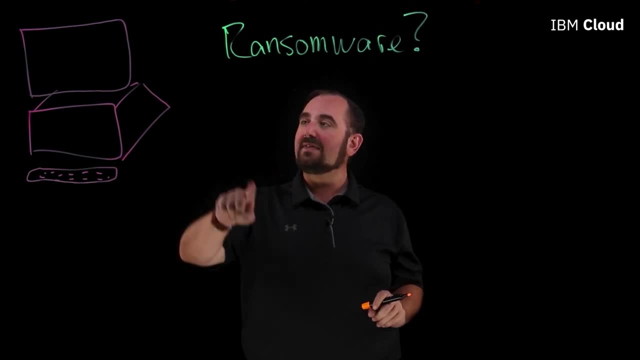 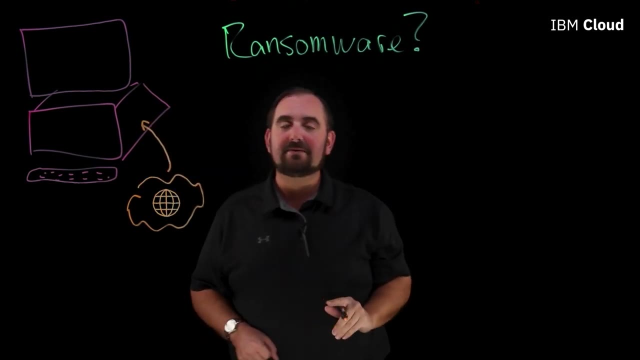 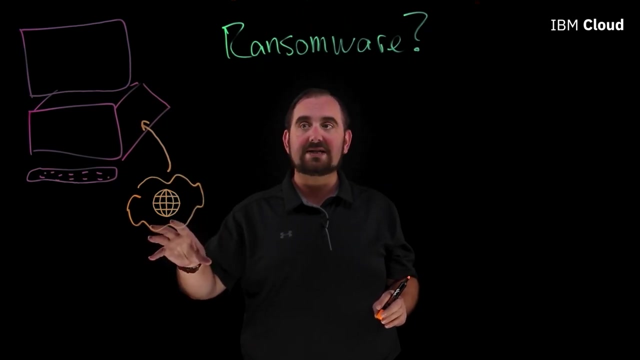 They're doing it to get paid. So what do they do? They take that vulnerability in your machine and they're going to transmit some software over the internet into the machine, and that software is then going to sit dormant and idle until it gets executed, And so it may have a time delay of a day, a week, a month, whatever, But there will be some sort of a time delay between when the malicious actor accesses the machine and when that code executes. 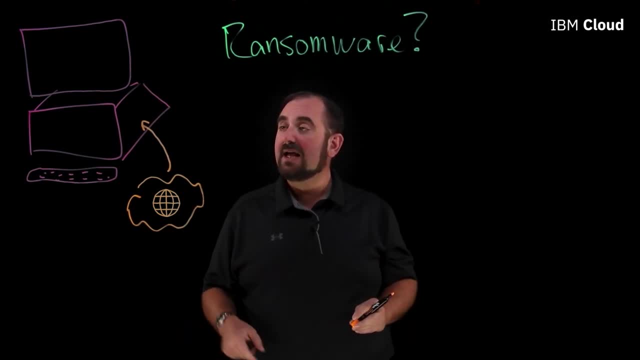 Now what happens? What happens when the code executes? The answer is that code is going to encrypt a very large proportion of the files on the machine. Now, what is it not going to encrypt? It doesn't encrypt the core operating system files, because if it does, the second part won't work. So it's going to encrypt all of the data that's not necessary to boot the machine up and get it running. So if it's a Windows machine, it's going to encrypt everything that's not in the Windows directory. 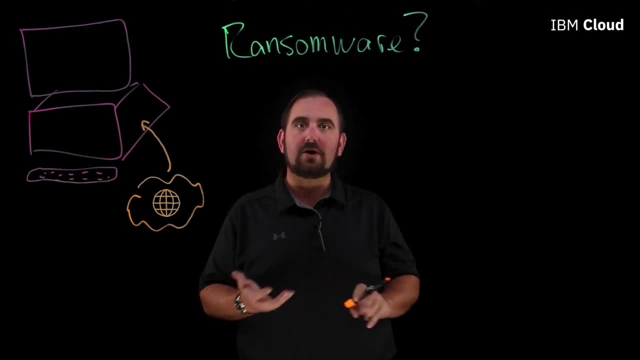 It's going to encrypt all of the games, all the spreadsheets, all of the files, all of the pictures, all of the everything on that machine. And then it's going to pop something up on the screen that's going to say: you've been hacked, you've been owned, your machine is compromised. 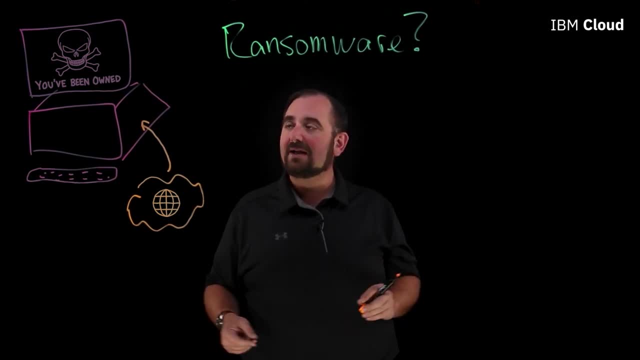 And the only way to get your data back is to pay a ransom- that's the ransom part of ransomware- to the malicious actor that has encrypted your machine. That ransom is almost always paid via a cryptocurrency Of some kind that has to be transferred to the attacker's wallet. 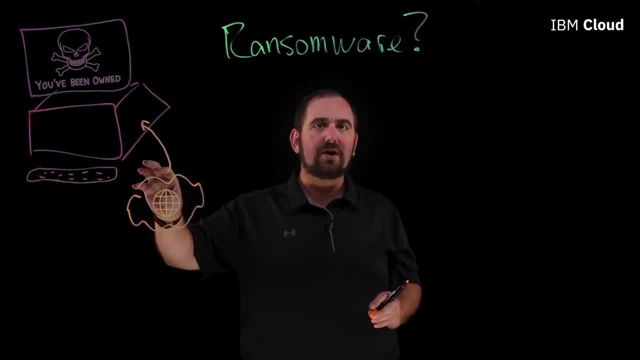 And so what I've just described is how it works on a consumer-grade machine. but, frankly, everyone, it's exactly the same thing on a server or on a fleet of servers. So again, malicious actors scanning for code vulnerabilities. they're looking for problems. The difference being, since it's not a consumer-level machine, they're in servers themselves, so they're first looking for holes in your network security And then, once they can get around your network, or if they find machines that are exposed directly to the public internet, then they're scanning for vulnerabilities on the machines themselves. 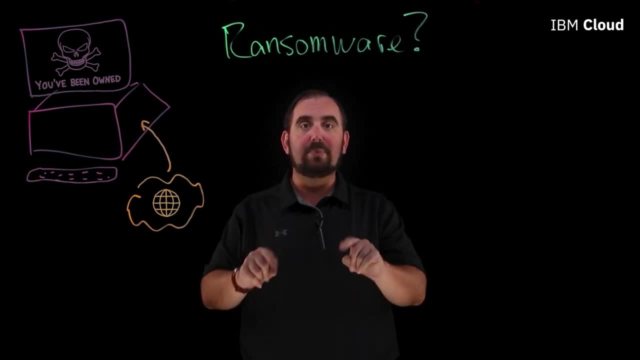 Again, they're looking for that exploit that nobody knows about. But let's be very honest here. the incidents of attacks using a zero-day or a previously unknown exploit are actually really, really, really small. The vast majority of these malicious actors are not using zero-day exploits. 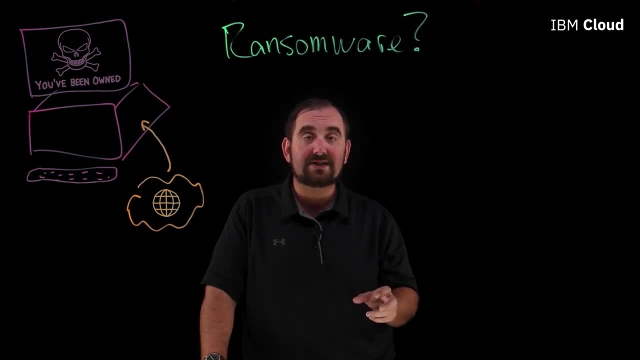 They're using exploits that have been known. Sometimes they're exploits that have been known for months or years, And so we're going to talk about remediation over here. Keep this point in mind, because it's a very important one. 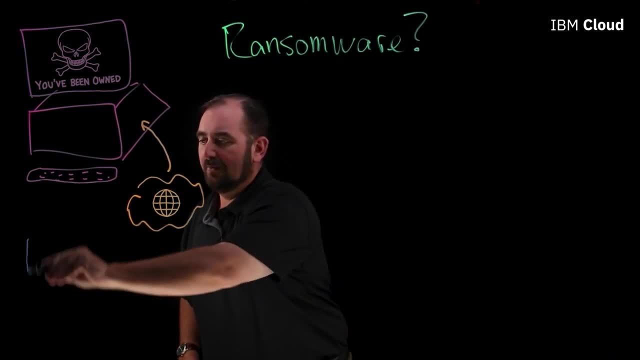 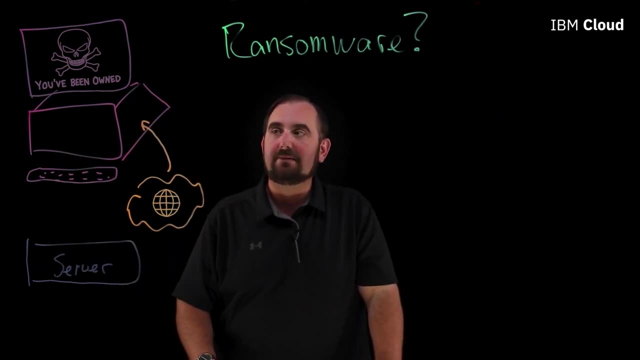 But back to our compromised system. So we're over here. we've got, you know, one or two or ten or fifteen different servers. The servers have been compromised. The malicious actor has spread through the network. He's gotten access to a number of servers in it. 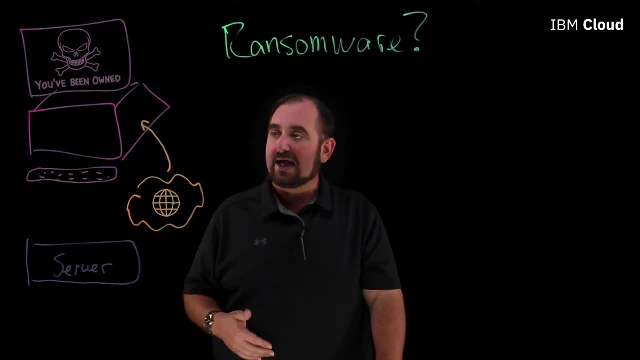 He's installed the ransomware And the only way to get any of that data back again is to pay the ransom. You have to pay the guy in hopes that he will send you the decryption tool that you need in order to get your data back. 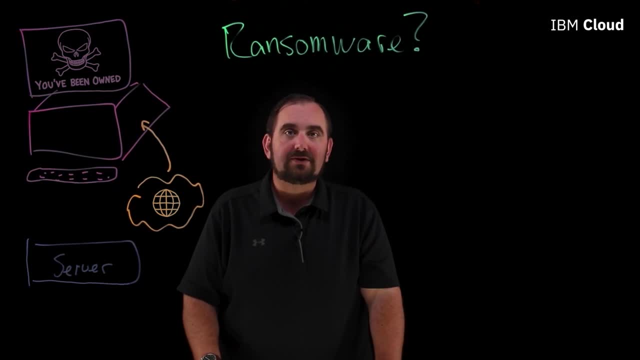 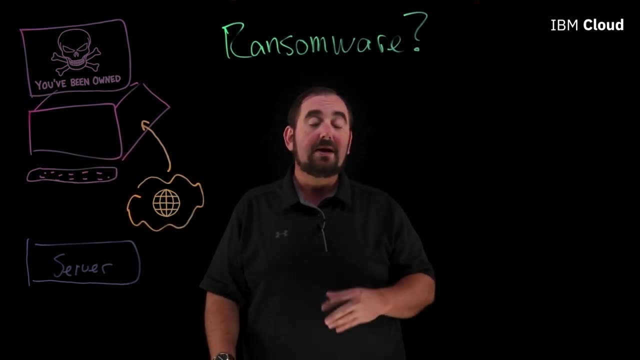 Now as to whether or not you pay the ransom, no one can answer that question for you. Hopefully, you have sufficiently prepared yourself that you never experience this to begin with, But if you do experience it, only you can answer the question: do I pay this ransom or not? 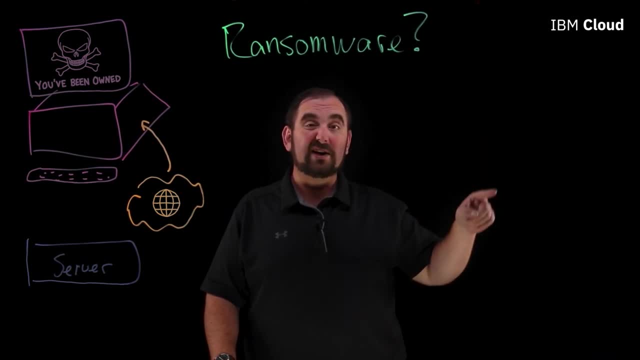 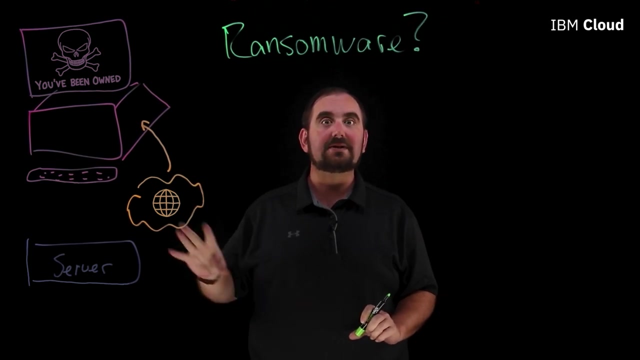 Now there are ways to avoid it, And that's what we're going to talk about next. So you have been owned. Worst case scenario. Now let's get into how do we keep ourselves safe? All right, So, in order to avoid letting those malicious actors, letting those hackers, get access to your system, 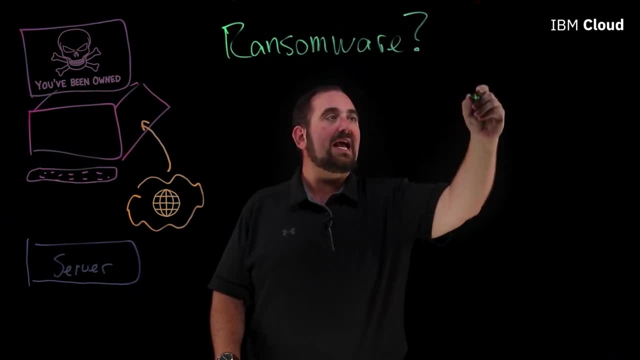 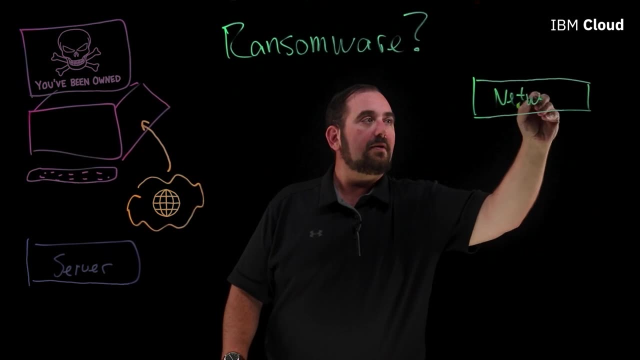 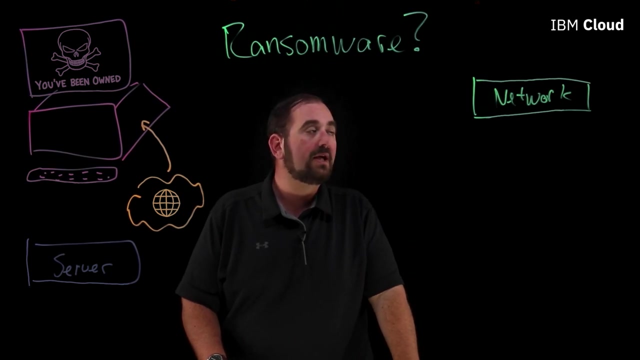 the first and most important thing you can do is have good network policies. It all comes down to the network. This includes both your home network and any kind of an enterprise or commercial network. If your network is properly set up, it is configured. 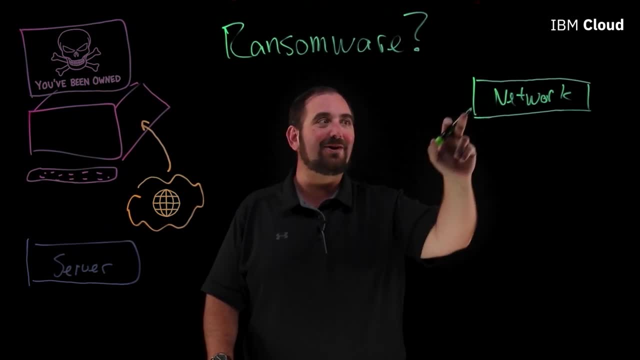 If you are regularly installing all of the patches and all of the firmware upgrades in order to keep your network equipment up and running safely. that is your first line of defense against any kind of a malicious actor getting into your machine. Second line of defense: 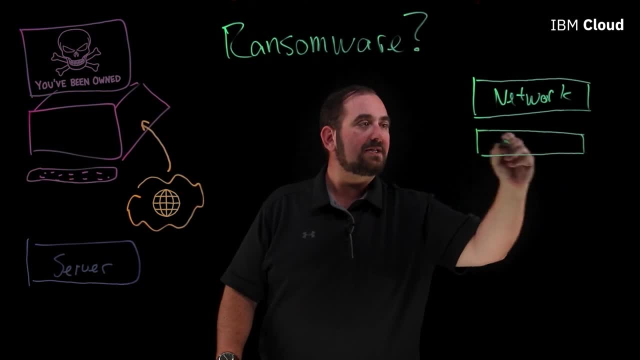 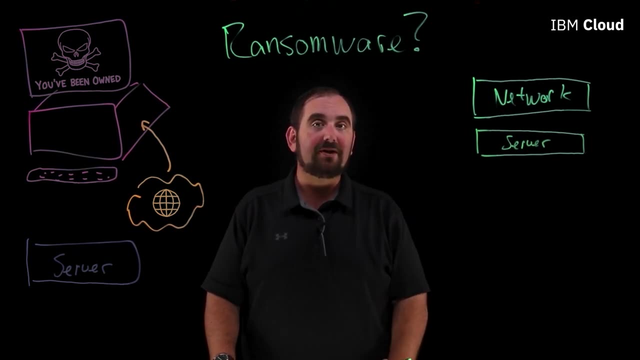 Once you get to the physical machine itself. So let's get to our- you know- server. here You must follow proper security protocols and practices to secure your servers. This is so, so, so important, And this goes beyond just user access control. 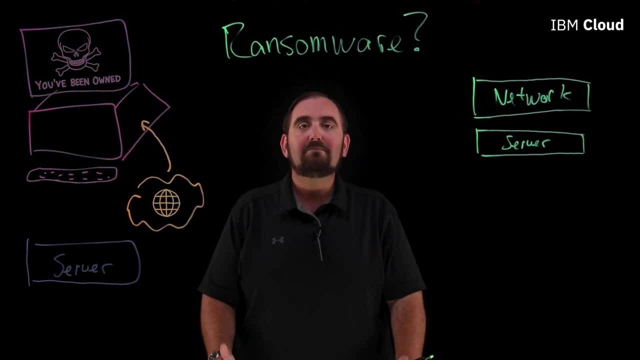 Although obviously user access control is incredibly important, Please don't ever use default passwords for anything. Please always use secure passwords. If you must use a password, use keys if at all possible. A key management system is superior to a user password in every possible manner. 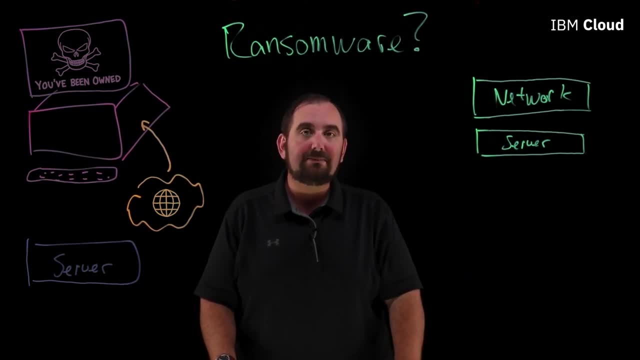 In addition to using keys, you must keep your machines updated. Software patches, hardware firmware patches are constantly being released. They are protecting you against these malicious vulnerabilities And, like we talked to a minute ago, the majority of these bad actors are using exploits that have been known for a while. 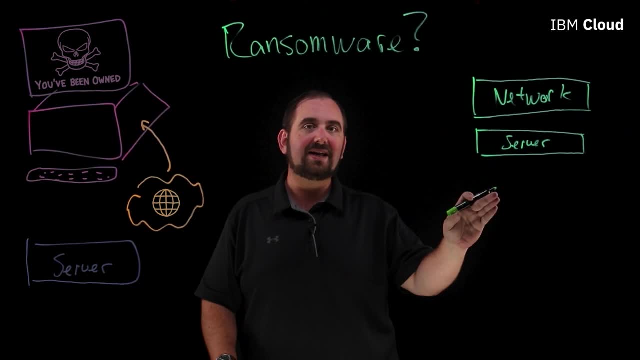 If you are on the enterprise side, if you are not regularly checking the CVE for vulnerabilities in the systems you run on a regular basis. you have got to add that to your best practice. You've got to do it on a regular basis If you don't have the time or the money or the staff to do it on your own. 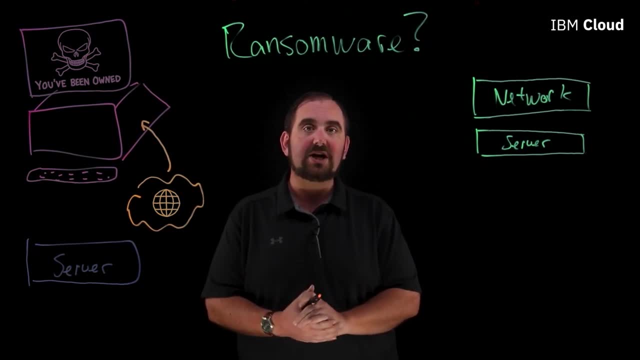 please engage with a vendor that is going to constantly be checking your systems, all of the operating systems and as much of the software as you run against that CVE list. You have to be checking it and you have to be getting things updated, Just because it's annoying to take some downtime to update firmware and update software. 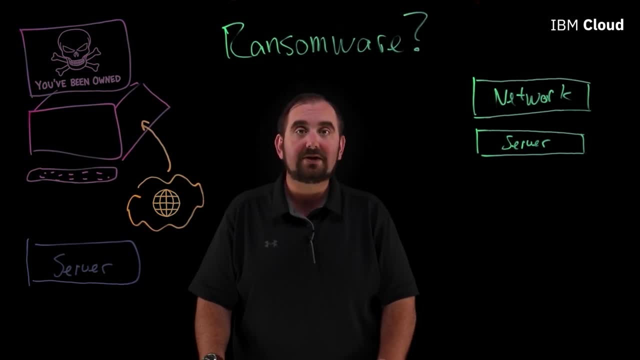 on those servers doesn't mean you can ignore it. Don't put it off. You have to keep these things modern and current. Don't run old versions of operating systems. And if you absolutely have to run an old version of an operating system, 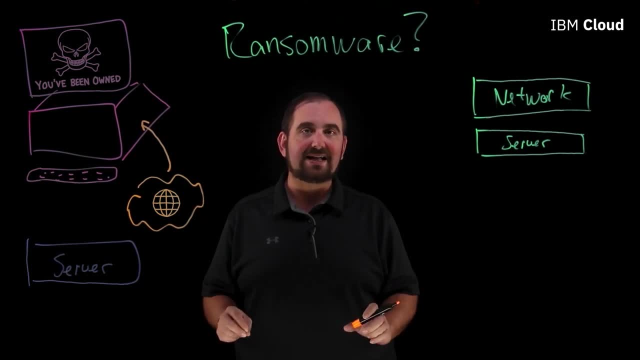 air gap the system, Make it impossible to access that system from the public internet. It is not safe to leave old Windows machines connected to the public internet. They will be compromised. There's just no other way around it. So please use modern hardware. 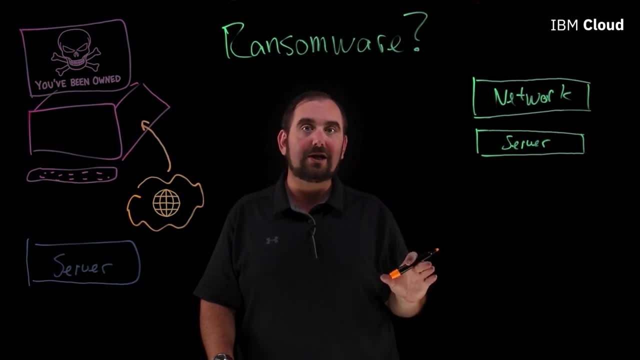 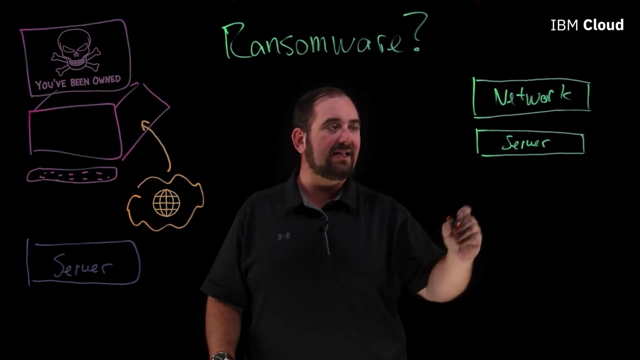 Use modern software. Keep all of your security patches and your firmware patches up to date. Next piece: Let's assume that you have a malicious actor. that's a little better than most, and they have found a zero-day vulnerability, a previously undisclosed vulnerability, one that's not yet on the CVE list. 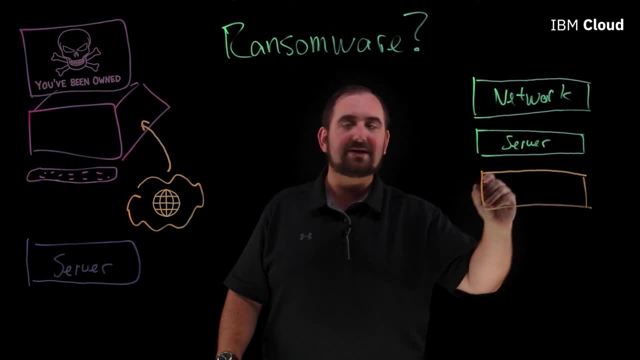 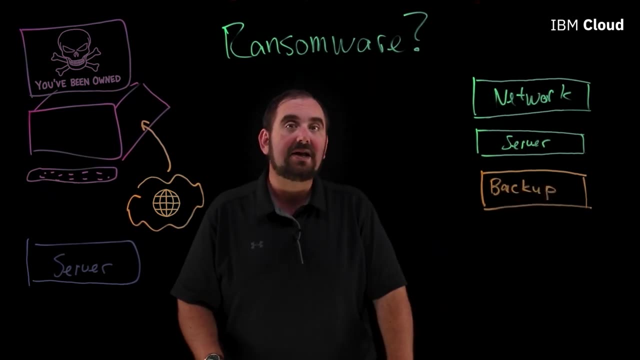 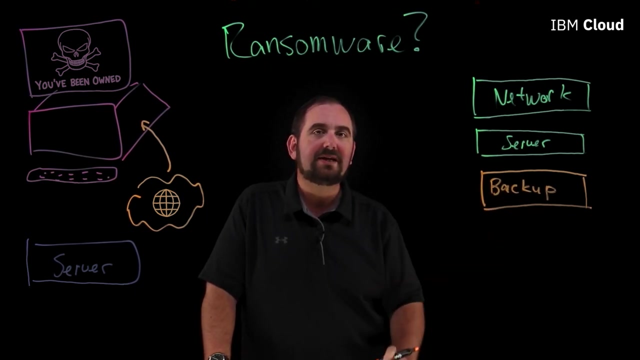 And this is one of the more interesting topics- You must back up your machines Now. back up your store is not the most fun thing to do On the planet- As a matter of fact, there's nothing fun about it- But if you are not regularly testing your backups for your ability to restore, 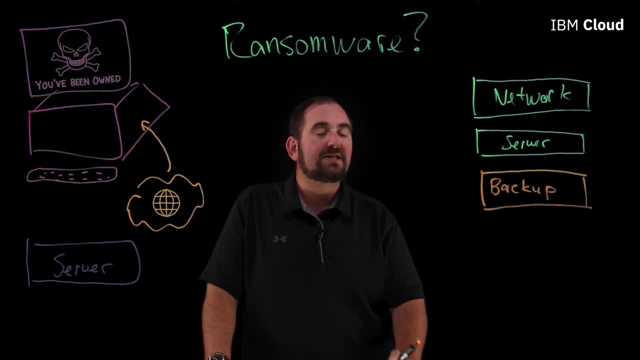 from them. you don't have a backup strategy. You must test those backups all the time. Once a year is not often enough. These backups are your only way to get back up and running if you've been compromised. It's the only way you're going to get back up without having to pay a ransom. 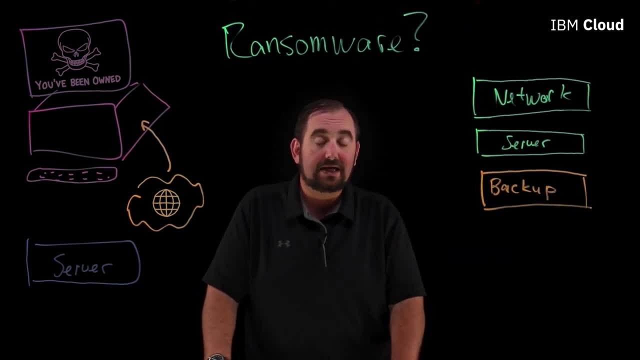 If you're a home user, the backups are how you're going to get your photos back. That's, I mean just frankly, you're going to lose whatever has been compromised, Whether or not you pay that ransom in many cases, because the decryption tool may not work. 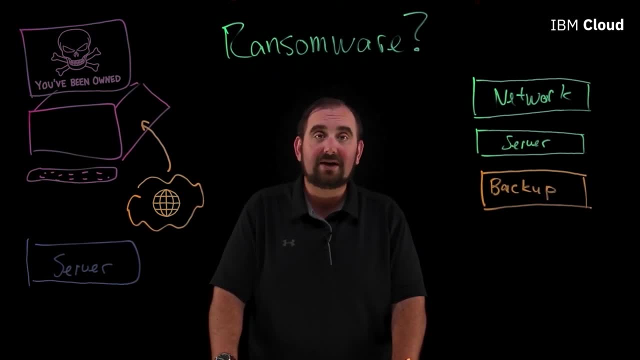 or this particular malicious actor may not care. They may just take the money and run. They have no obligation to provide you with what you've paid for. Again, they're criminals. This is how they get started in the first place. So have a backup strategy, have a restore strategy, have a good network map of all. 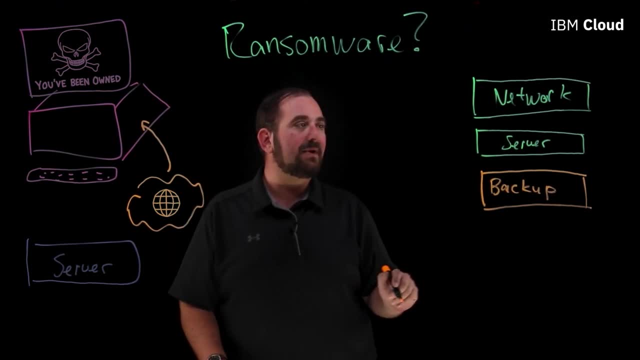 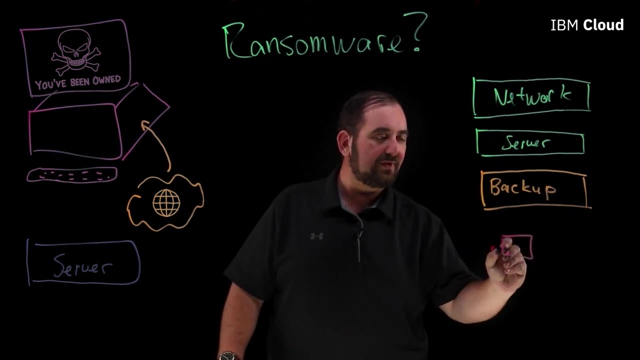 of your systems and their interconnections, because if somebody can compromise one server, they can probably compromise multiples. And so let's imagine here our enterprise network, Right? So we've got server here one, and we've got, you know, an Active Directory server over here. 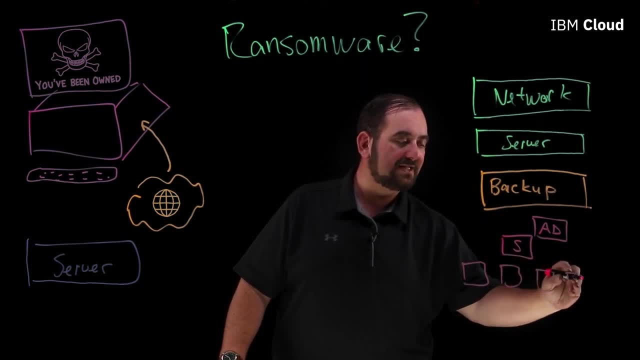 And we've got servers- you know, three, four, five, six, seven, whatever, So on and so forth. Everything is all interconnected. Right, Active Directory is going to get all of the controls. Let's say that the server that gets compromised is your Active Directory server. 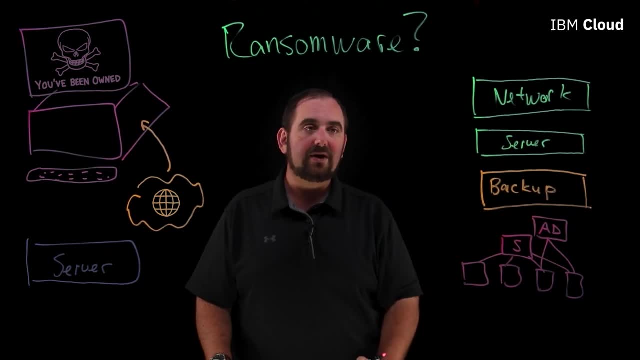 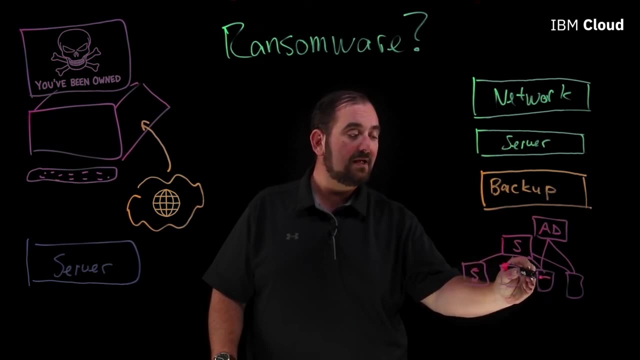 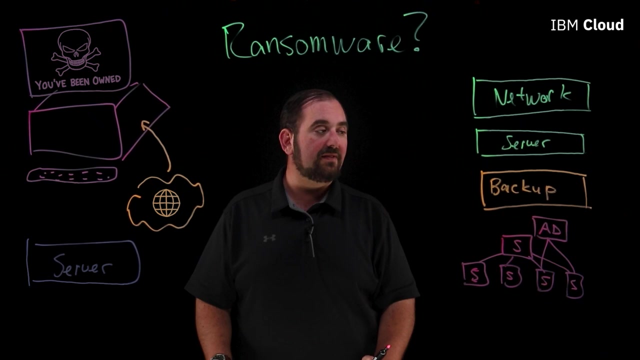 This is kind of like worst case scenario stuff here. Once they're into your Active Directory server, if they can get some credentials, they can start getting into everything else that you have running in your environment. they're going to compromise everything, And so once they have compromised it, once they have encrypted everything, 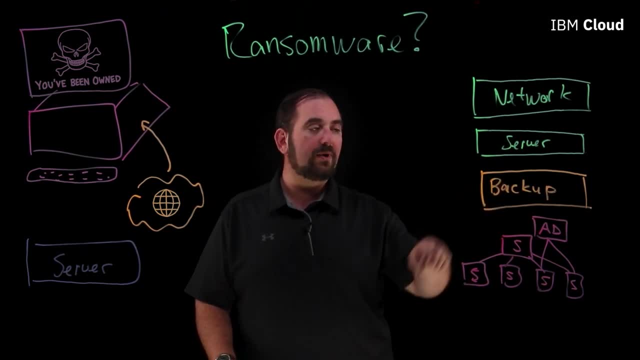 they've sent you their ransom message. you then have to make the decision. All right, Are we going to try to restore from a backup? Well, remember at the beginning when I said that the malicious actor they were going to install code. 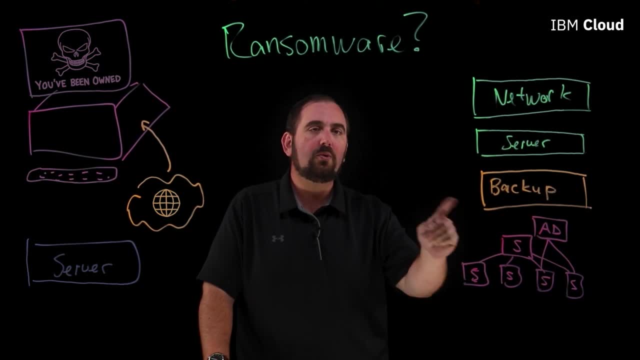 but they weren't going to trigger it yet. Do you know when you were compromised? Because you have to restore to a backup that exists before. you were compromised. Because if you restore a backup, your backup strategy is great. You've got good systems images. 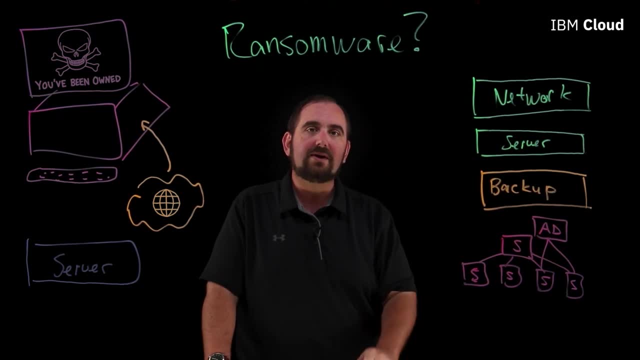 You can bring everything back from a backup from last week, But oh wait, you were compromised six weeks ago. All you're going to do is you're going to restore good backup copies that still have the malicious code in them. If that's the case, do you have the ability to find? 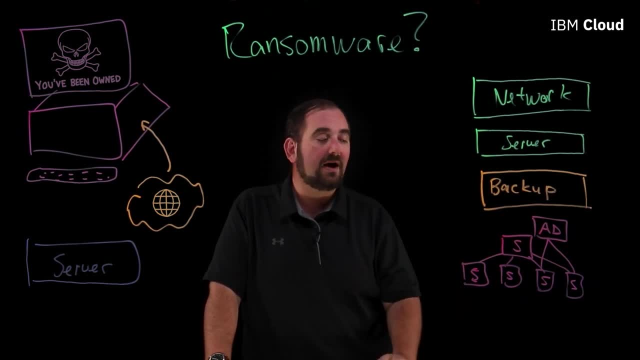 that malicious code and eliminate it before it activates itself again. Otherwise you're going to find yourself in exactly the same spot: No access to systems, no ability to process workloads, no ability to run applications. You are down. So that is what ransomware is. 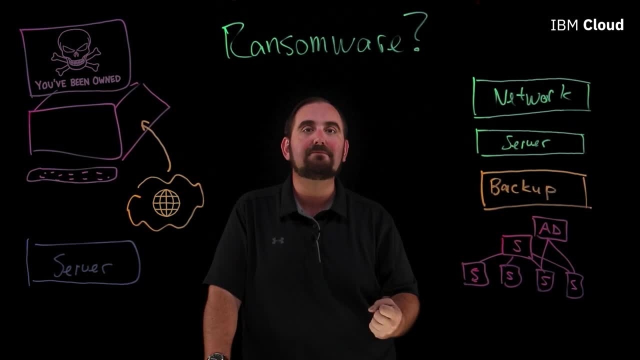 These are some ways to protect against it. Please, please, please, I implore you, learn about ransomware and learn how to protect yourself against it. Engage companies that have expertize. you know folks that know a lot about CVE, folks that know a lot about network security, that know about secure server. 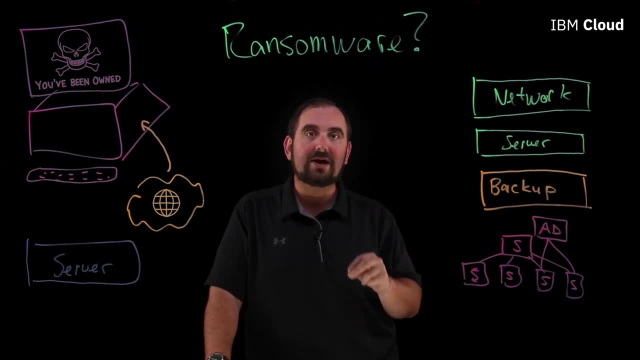 security. engage with your operating system vendors to be sure that you're on a regular patch and maintenance cycle, to be sure that you are protecting yourself against these kinds of attacks. Hopefully you found the information today valuable. If you have any questions, please feel free to leave them in the comments and we'll talk to you later. 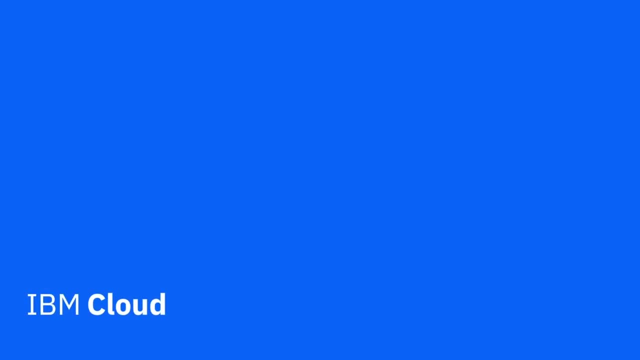 Thank you so much for stopping by the channel today. If you have any questions or comments, please feel free to share them with us below. If you enjoyed this video and you would like to see more like it in the future, please do like the video and subscribe. to us, so that we'll know to keep creating for you.